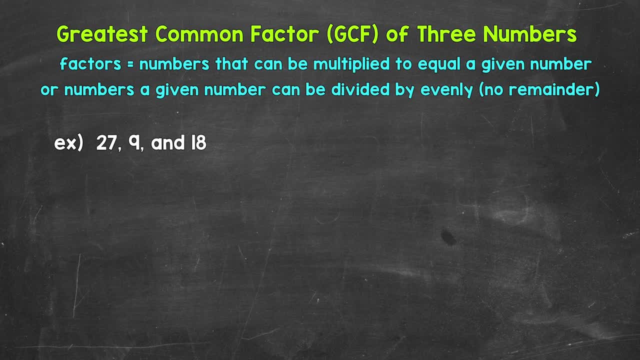 and then find the greatest common factor. Let's start with the factors of twenty-seven Now. I would suggest always starting with the factors of one and the number itself, because we know one times that number will equal that number itself. We can think of factors in terms of pairs. 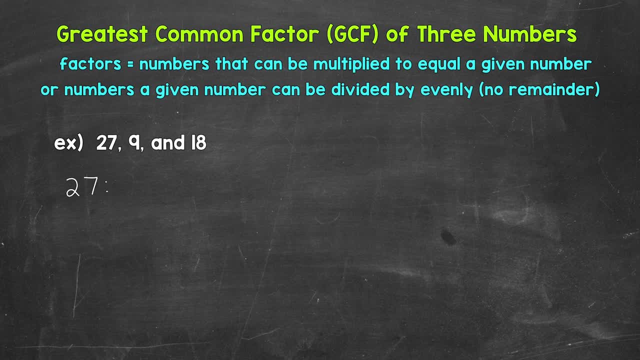 One times twenty-seven equals twenty-seven, Or we can divide twenty-seven by those factors, evenly, However you want to think about it. So I'm going to write one and twenty-seven with a gap in between for the other factors. That way we can write the factors in order. 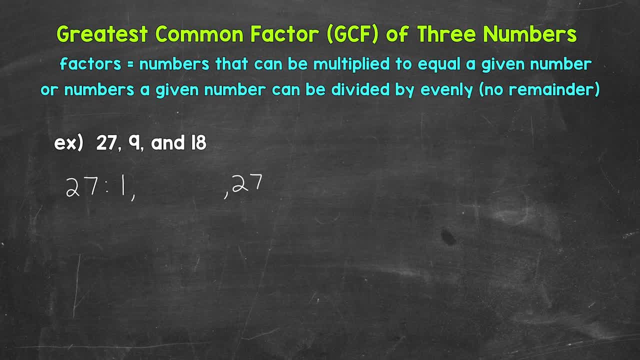 Now we need to list the other factors of twenty-seven. So let's think about what else goes into twenty-seven, so to speak. Think about multiplication facts, division facts, and we can work our way up from one. So there are different strategies and ways to work with this. 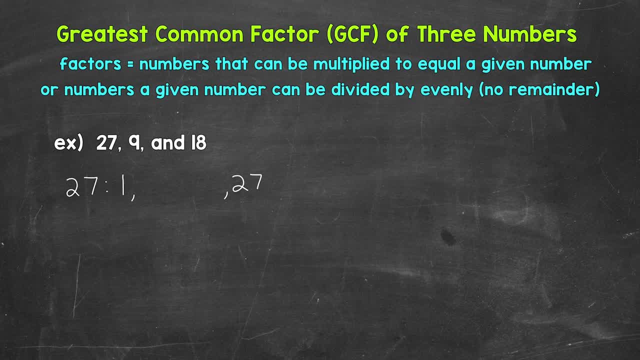 So there are different strategies and ways to work with this. So there are different strategies and ways to work through this. The next factors of twenty-seven are three and nine. Three times nine equals twenty-seven, so three and nine are factors of twenty-seven. 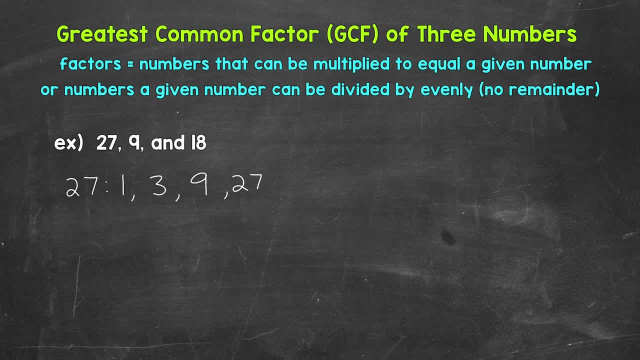 And that's actually it for the factors of twenty-seven. You can always think about other possible factors if you're unsure, if you're done. for example, two, four, five, six. for example: two, four, five, six. 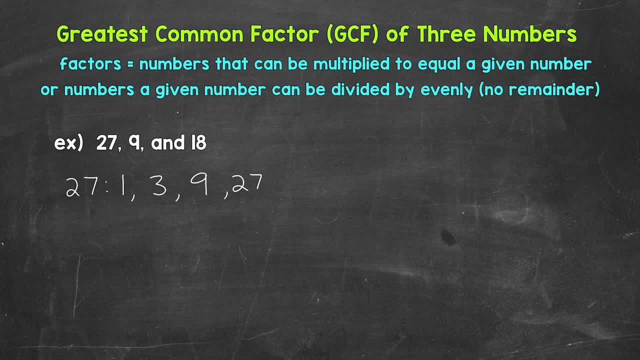 and so on, But we have them all: 1,, 3,, 9, and 27.. And, like I mentioned earlier, we can also think of these factors in terms of division. We can divide 27 evenly by all of these factors. 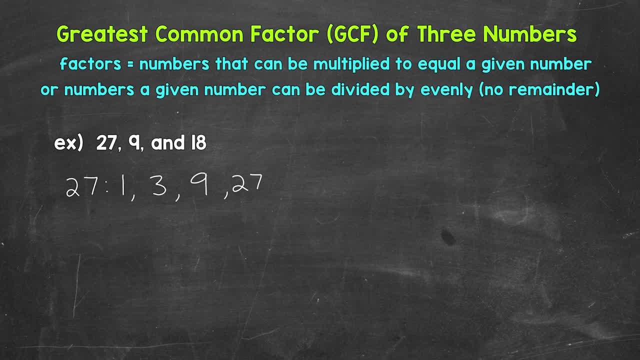 Now, one thing I do want to mention about factors and writing out factors lists is that you will get a lot better the more you do Everything from writing and recognizing factors to the spacing of your lists. So something to keep in mind. Let's move on to the factors of 9. And we can start with. 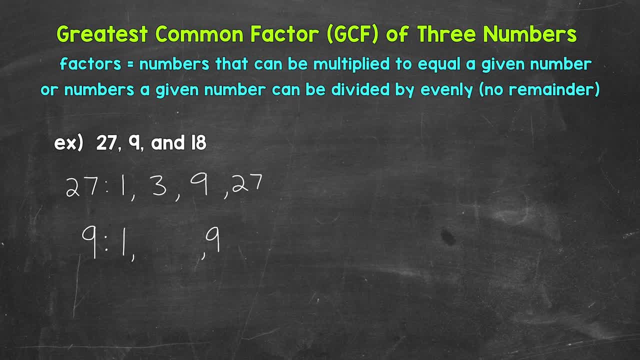 1 and 9.. Now we need to think of other factors of 9.. Well, 3 times 3 equals 9.. So 3 is a factor of 9.. 3 equals 9.. And although 3 is a factor of 9,, 3 equals 9.. 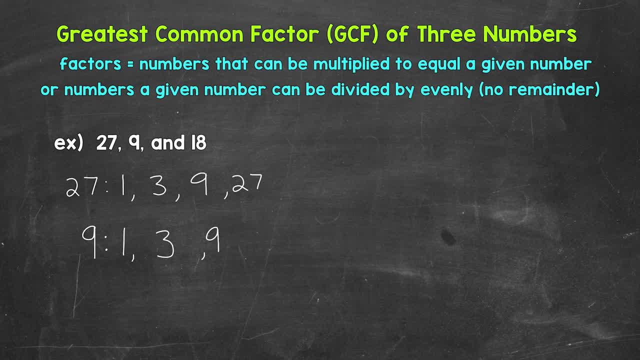 And although 3 is a factor of 9,, 3 equals 9.. 3 times 3 equals 9.. We just need to put 3 once there. as far as the list of factors. Lastly, let's list the factors of 18.. 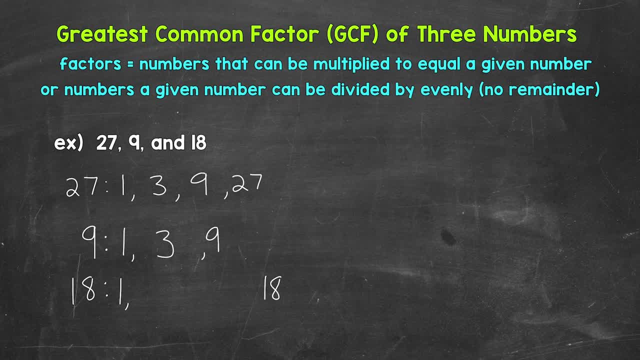 We can start with 1 and 18.. Next we have 2 and 9.. 2 times 9 equals 18.. So 2 and 9 are factors of 18.. And then, lastly, we have 3 and 6.. 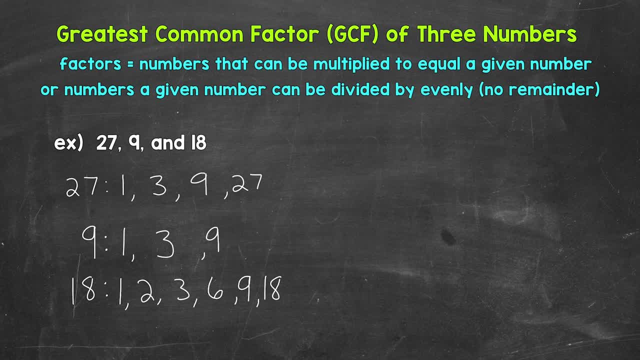 3 times 6 equals 18.. So 3 and 6 are factors of 18.. And that's it for the factors of 18.. 1,, 2,, 3,, 6,, 9, and 18.. 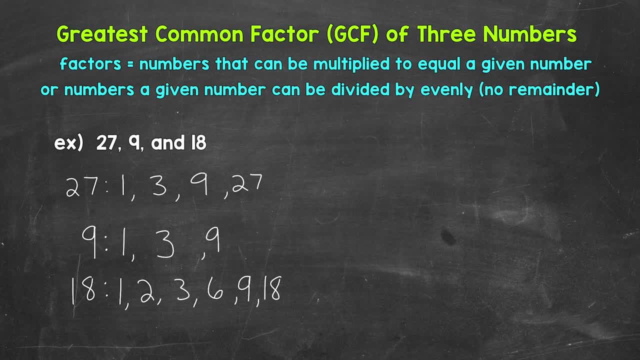 Now that we have all of the factors listed for our numbers, we need to look for common factors, so factors they share, And then, specifically, we need to look for the greatest common factor, So the greatest factor in value that they all share. 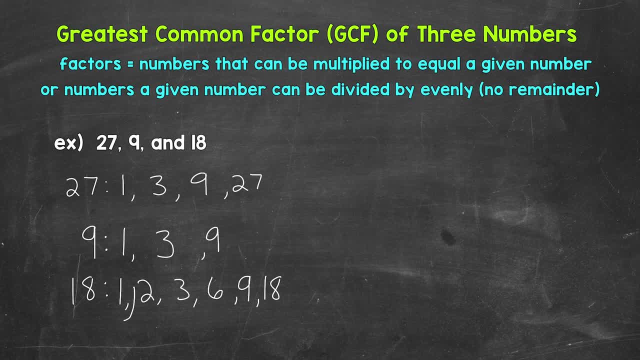 that they all have in common. So 1 is going to be a common factor, 3 is going to be a common factor And then 9 is going to be a common factor. So there are 3 common factors between these numbers. 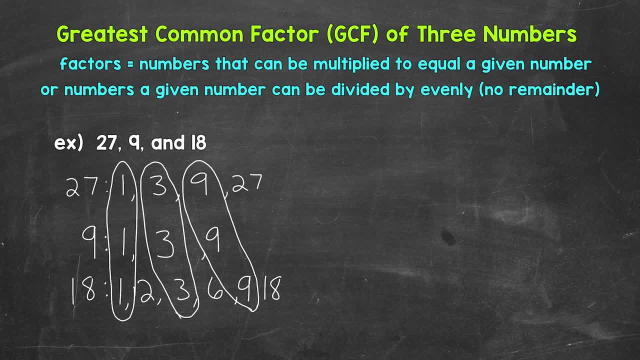 Now the greatest common factor is going to be 9.. So over to the right I'll write: the GCF, which stands for the greatest common factor, equals 9.. So the greatest common factor of these 3 numbers- 27,, 9, and 18, is 9.. 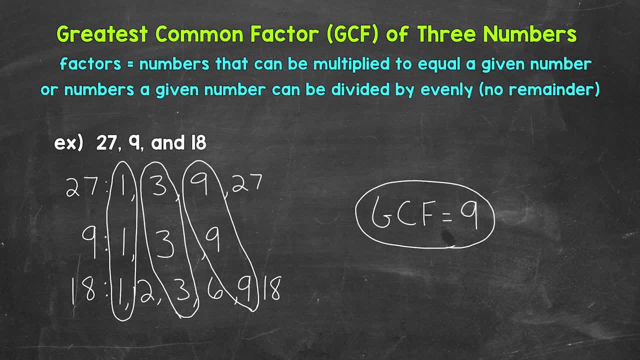 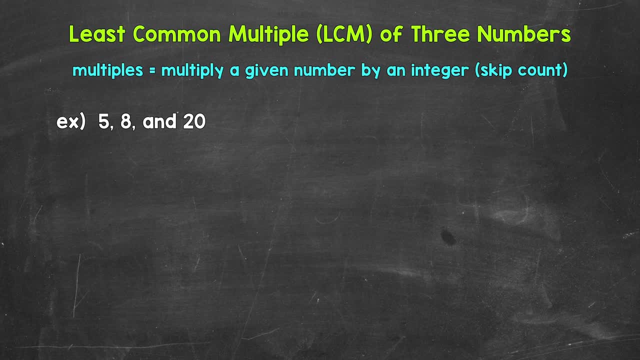 So there's how we find the greatest common factor of 3 numbers. Let's move on to the least common multiple of 3 numbers. Here is our example for the least common multiple of 3 numbers And just like we talked about with the greatest common factor of 3 numbers, 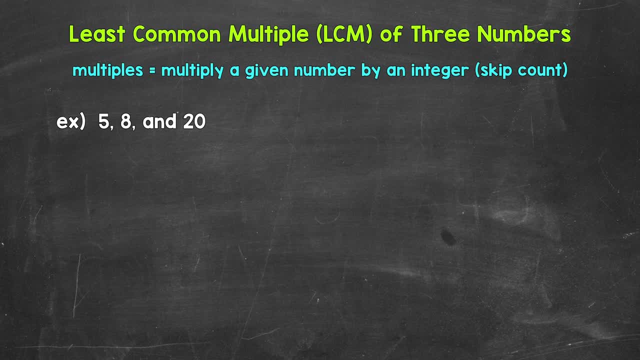 this is going to be the same exact process we use for 2 numbers. when it comes to the least common multiple, We just have that extra third number. Now, a multiple is the result of multiplying a given number by an integer. When we think of the multiples of a number, 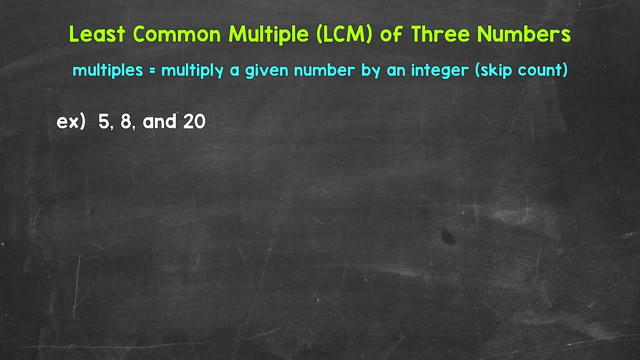 we need to think about the numbers we get when multiplying that given number by integers. A simpler way to think about multiples is to think about skip counting. So all of the numbers, something is going to hit when you count up by that number. Those are all going to be multiples. 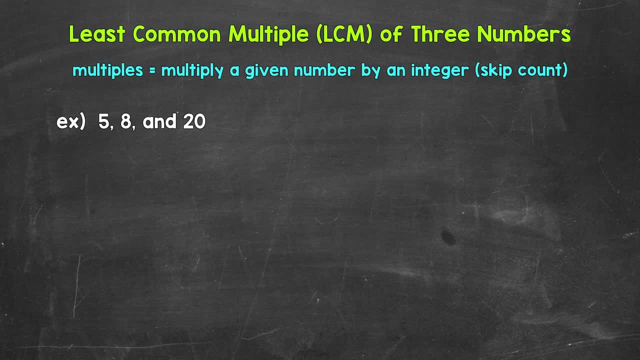 This will make a lot more sense as we go through our example. Let's jump into our example where we have 5,, 8, and 20.. So let's find the least common multiple between these 3 numbers. Let's start with some multiples of 5.. 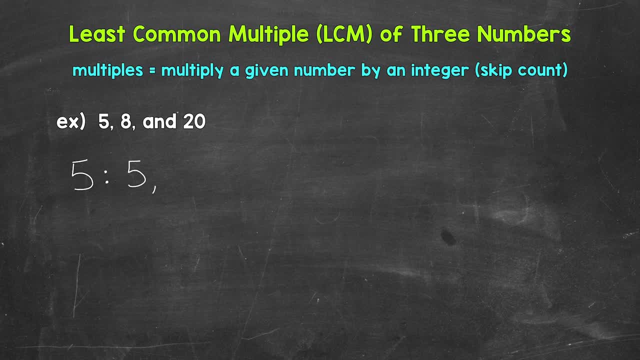 So 5 times 1 is 5.. 5 times 2 is 10.. 5 times 3 is 15.. 5 times 4 is 20.. And 5 times 5 is 25.. So you can see that we just skip counted. 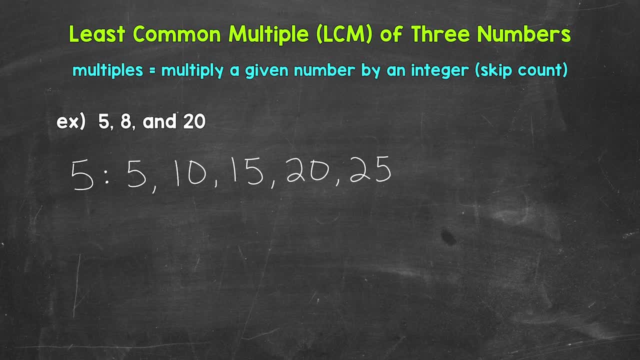 by 5 to list those multiples of 5.. 5,, 10,, 15,, 20,, 25.. So on and so forth. Now I stopped at 25, because multiples go on forever, They are endless, They are infinite. 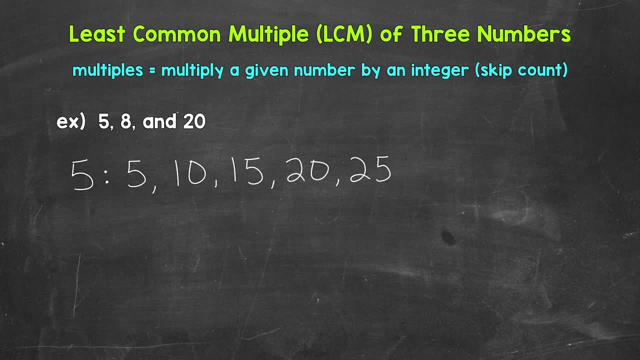 My suggestion is to list 4 or 5 multiples of each number when looking for the least common multiple. So list 4 or 5 for each number, Look for any in common, Specifically the least common multiple, And if you don't have any in common, you can always extend the multiples lists. Now let's list the first 5 multiples of 8.. 8 times 1 is 8.. 8 times 2 is 16.. 8 times 3 is 24.. 8 times 4 is 32.. 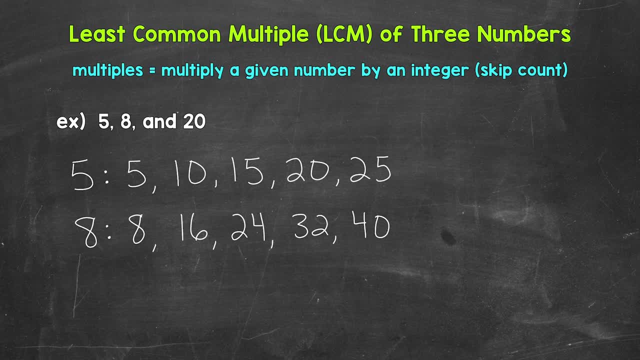 And then 8 times 5 is 40. So 8,, 16,, 24,, 32,, 40. So on and so forth. And then, lastly, let's list the first 5 multiples of 20.. So 20 times 1 is 20.. 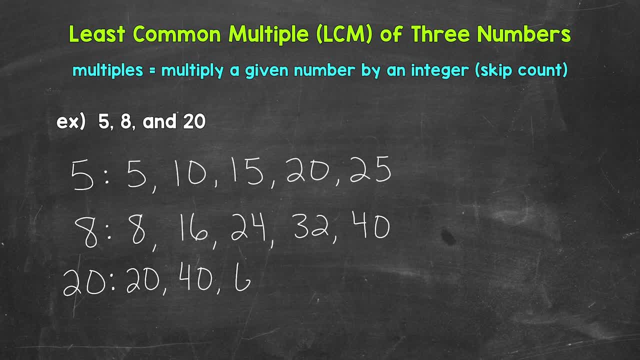 20 times 2 is 40.. 20 times 3 is 60.. 20 times 4 is 80.. And then 20 times 5 is 100.. So 20, 40, 60,, 80..